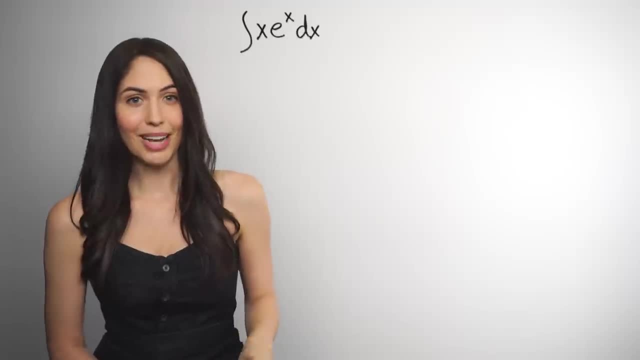 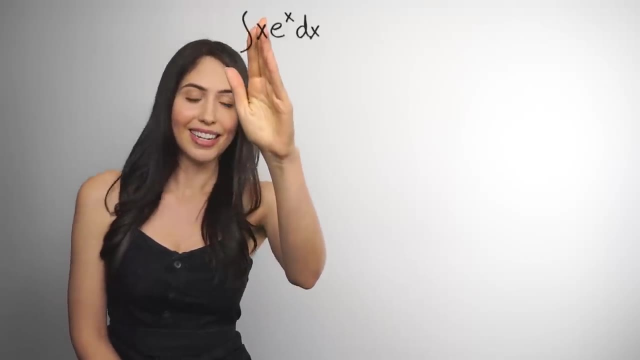 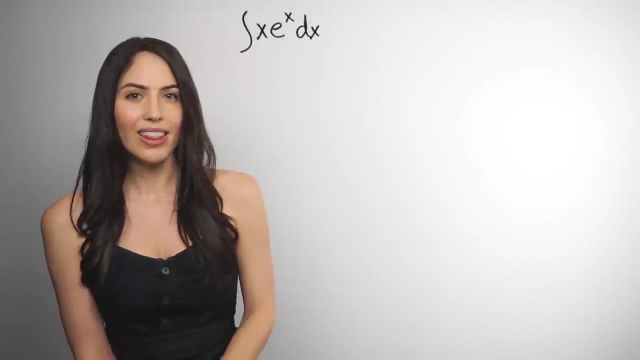 I mean, if this were just integral of x dx, you could do that easily. If it were just integral of e to the x dx, you could do that with the basic integration rules, which hopefully you've learned already. But it's not that We have the two of them multiplied together. 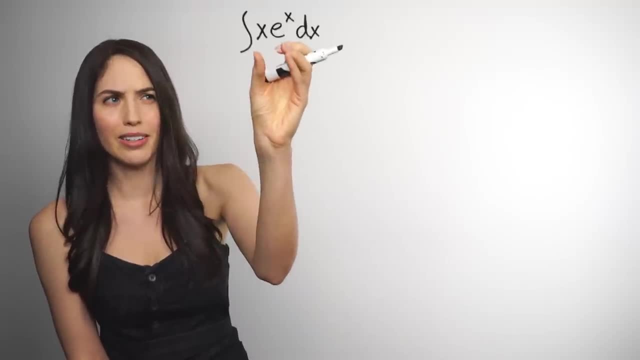 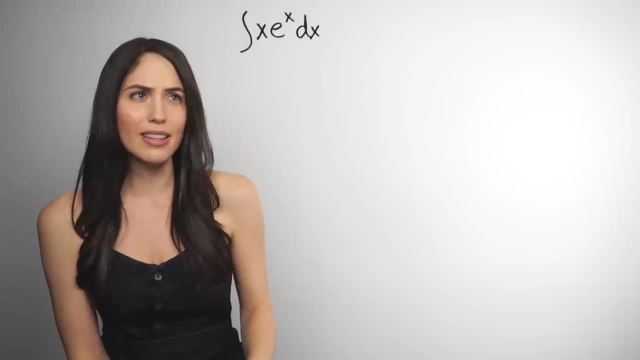 So you can do this. We have this product here, which makes it trickier. So what do we do? Well, first of all, quickly, you should check to see if maybe you can just simplify this with algebra, combine it and put it together. You can't do that here. I'm just saying it because sometimes 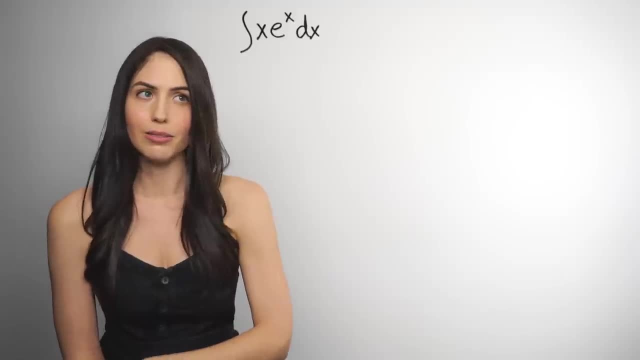 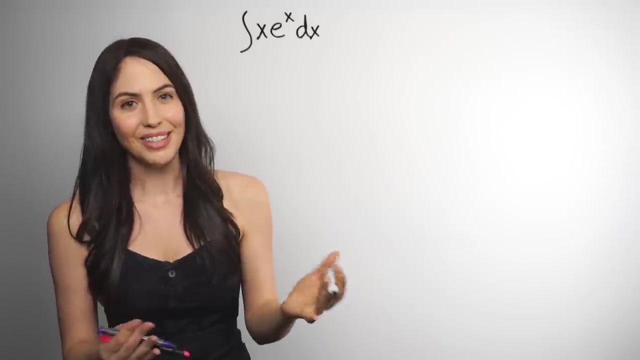 you can, and that would make it a whole lot better. but that would be too easy here. So what do we do? The next thing you try is a substitution, So a? u substitution. You should try it, See if it works. It works and helps. I'm telling you that, no matter what you choose for u, for the substitution, 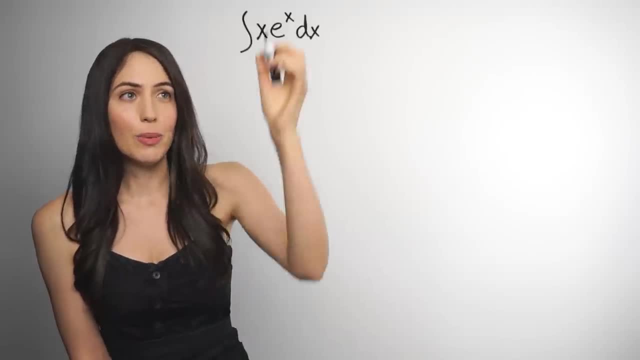 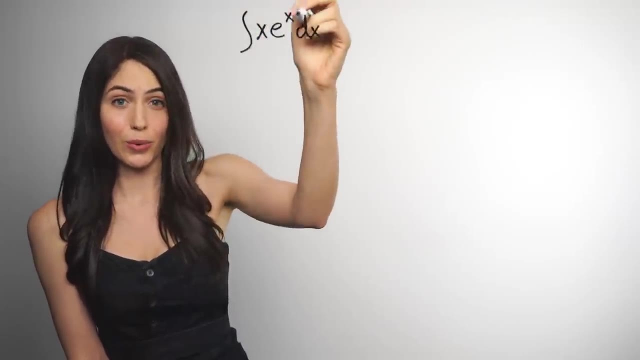 it's not going to make it integrable. Like, if you pick u to be x, your du won't be what you need to cover the rest of the integrand If this were x squared, then a u there would help, because this would be what you want for your du: the right order, power of x. But it's 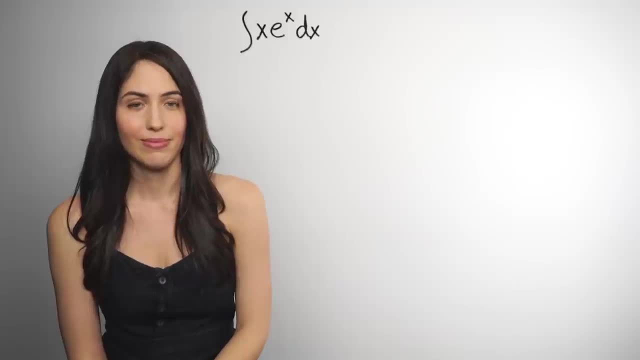 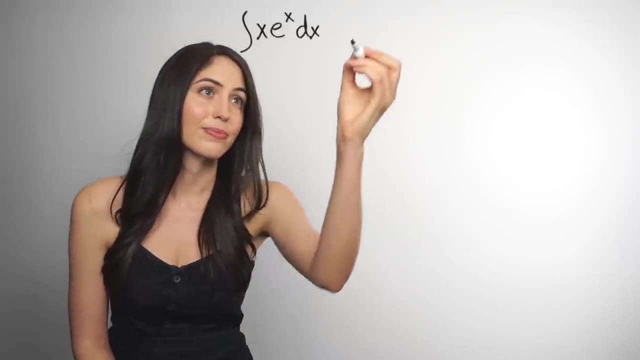 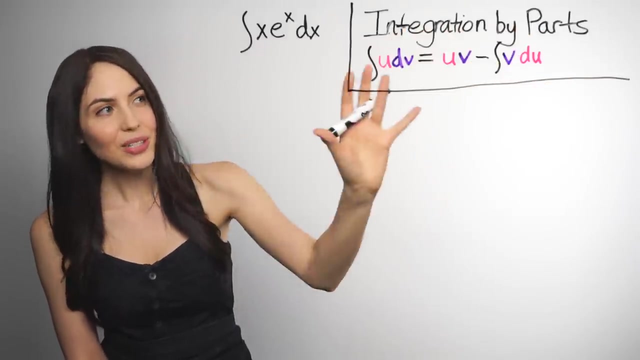 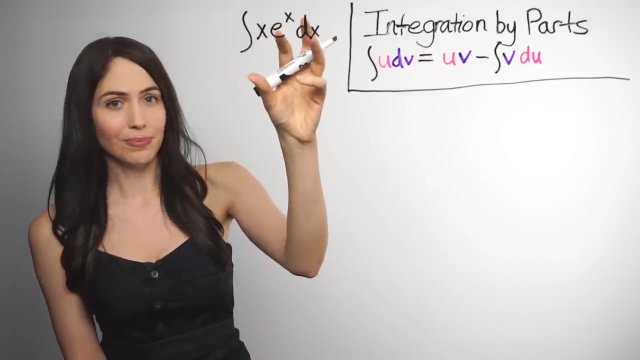 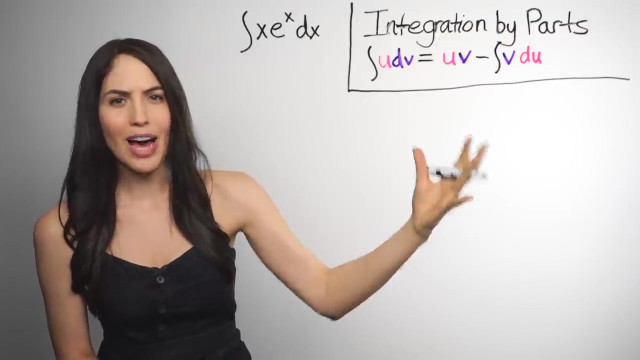 not, But you should try substitution first. And what do we do if all of our usual tricks won't work? Well, we need something new. This is the integration by parts formula. What is that? All it does is takes your integral and it rewrites it using a new, different, integral. Why would we do that? Because, hopefully, 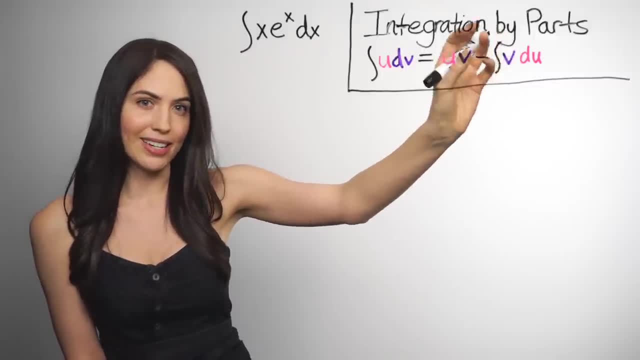 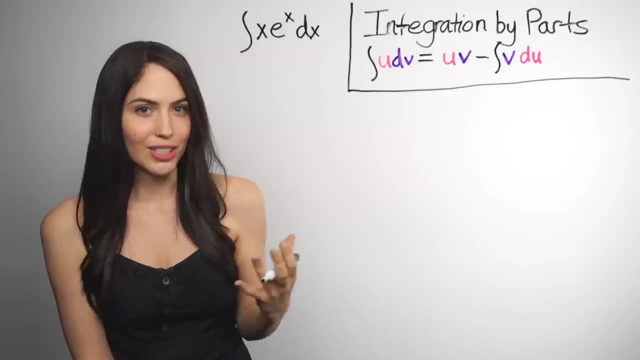 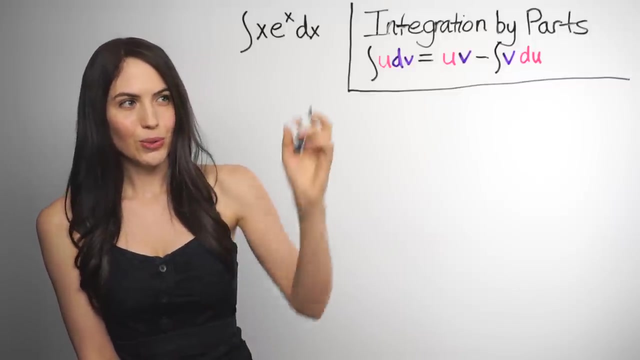 the new integral is easier to do, something we can integrate. So a lot of the work of integrating is whipping something into a shape where we can actually do it. So this sounds great. Wait, what's the catch? You have to choose what's u and what's dv yourself, and 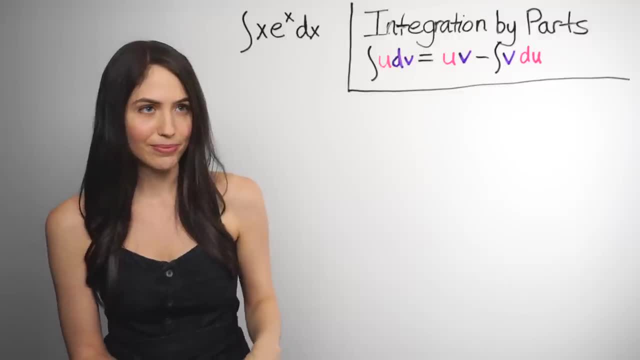 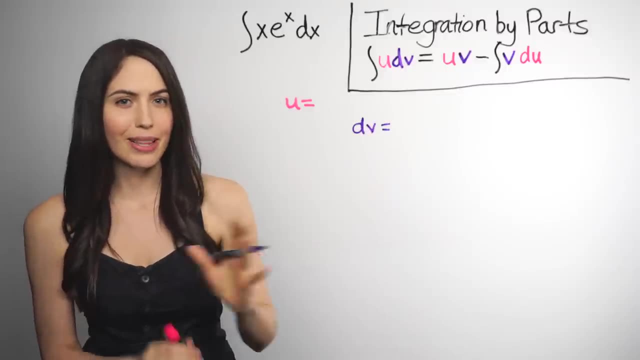 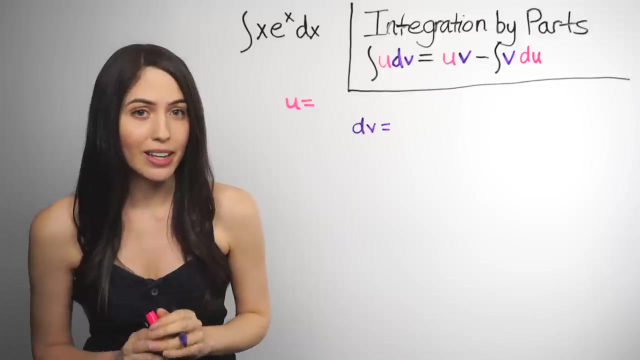 carefully in order for it to work. So choosing u and dv can be the most confusing part- the hardest part, I think. But don't worry, I'm going to show you how to do it And I'm going to show you a trick in a minute. 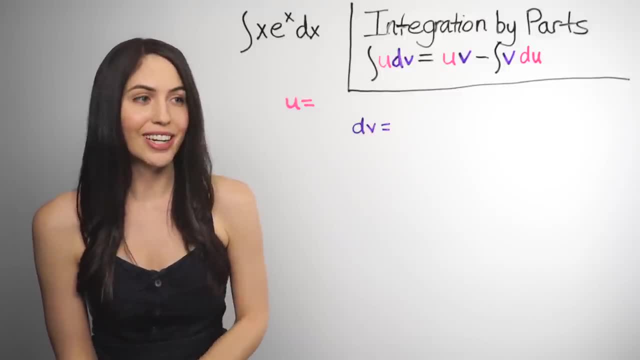 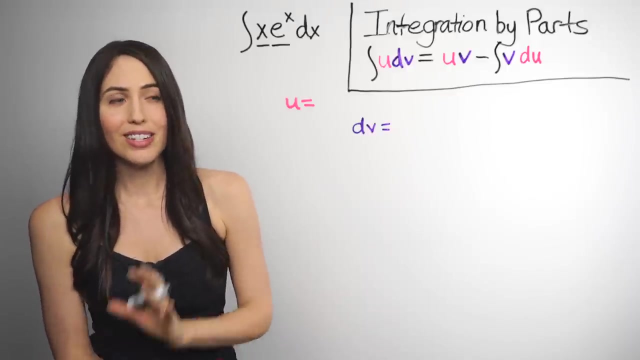 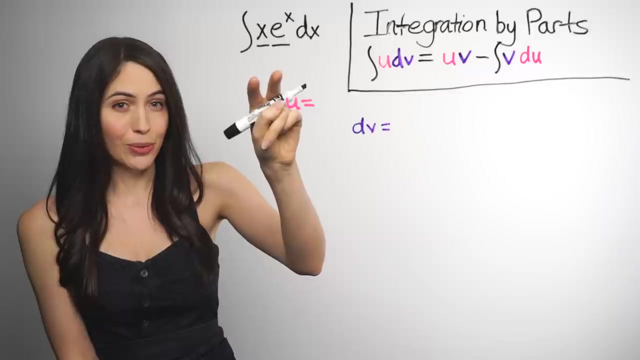 the LIATE acronym trick. But first here's the general idea, a good rule of thumb, And you're going to see a lot of different rules and mixed messages out there, But generally for this, whichever of your two factors gets simpler when you differentiate. it. make that. 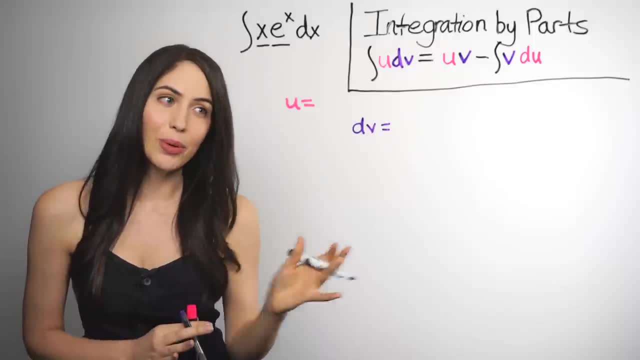 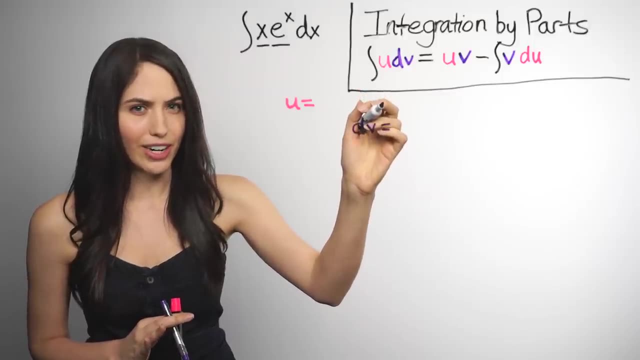 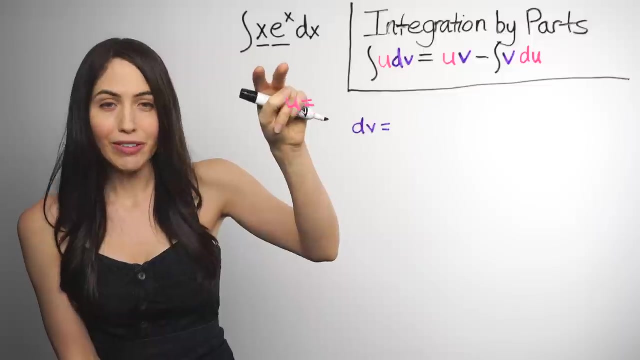 your u And then the other one will be your dv, unless that one would get more complicated when we integrate it, which doesn't happen a lot. But basically pick for u whichever of your two factors gets simpler, breaks down, gets smaller. 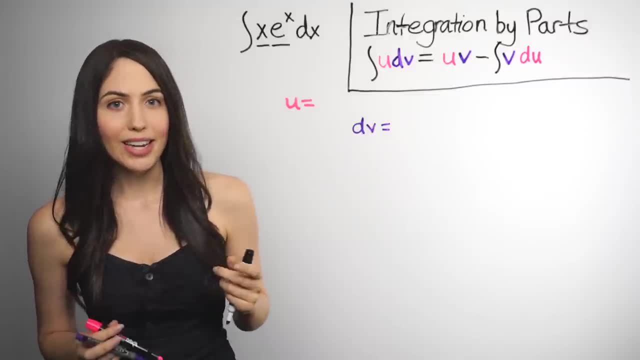 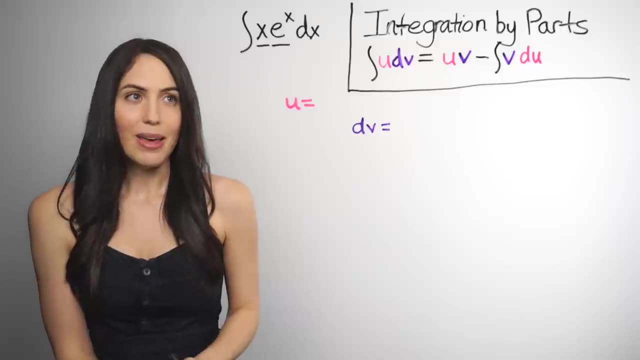 When you take the derivative of it. so maybe the degree gets smaller, the order of it gets fewer terms. If it reduces in some way, make that your u and then the other one your dv. And if this all sounds really confusing, that's because it is, So let me show you what I mean. 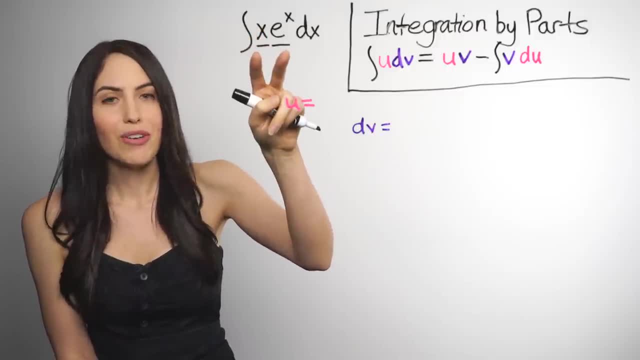 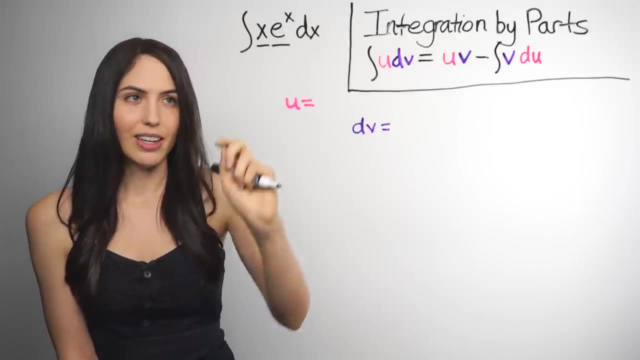 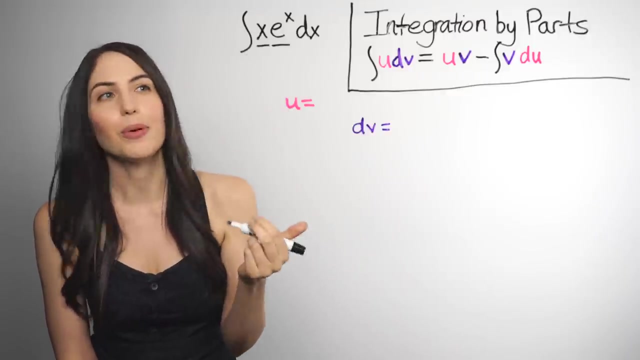 in this one. Which of our two factors, x or e to the x, gets simpler when you take the derivative of it? Well, the derivative of x is just 1.. That's simpler. The x dropped out, It's a lower order or degree or power. The derivative of e to the x is just e to 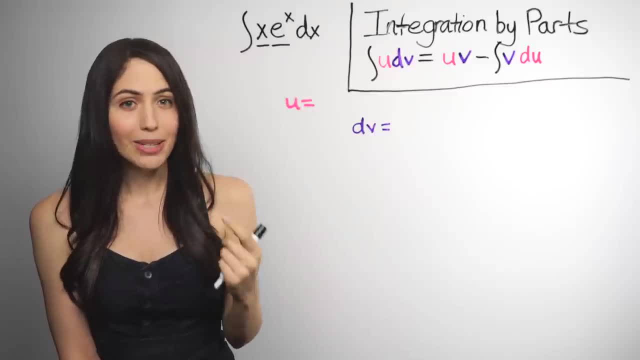 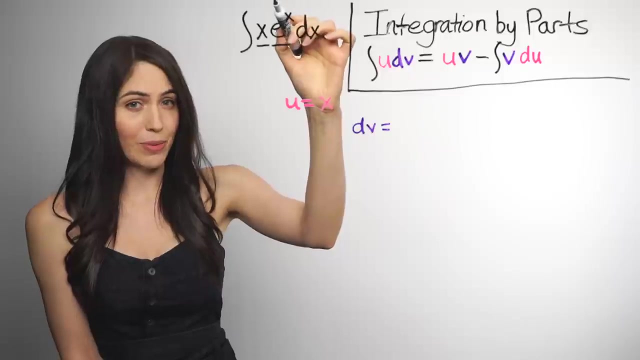 the x again, which is not simpler. So probably our u is going to be x And then the other factor, e to the x, should be our dv, Unless e to the x is going to be our dv, And then our dv will get more complicated when we integrate it, which it doesn't because the 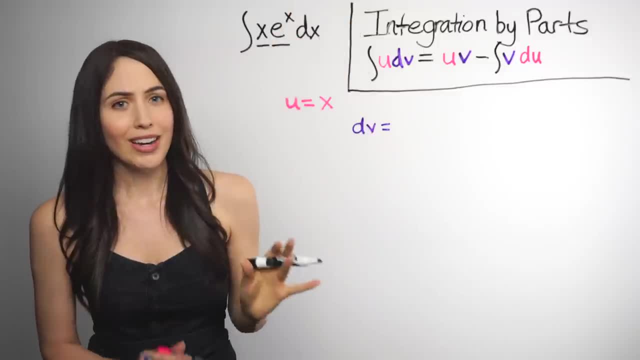 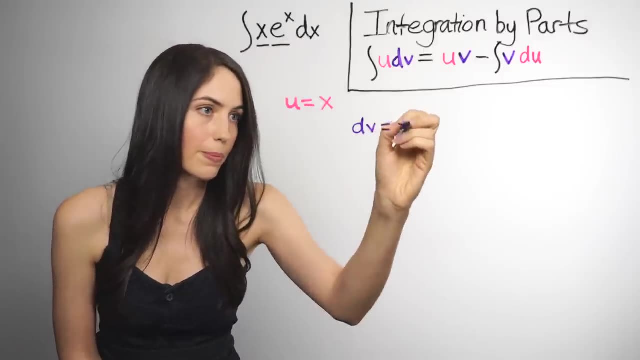 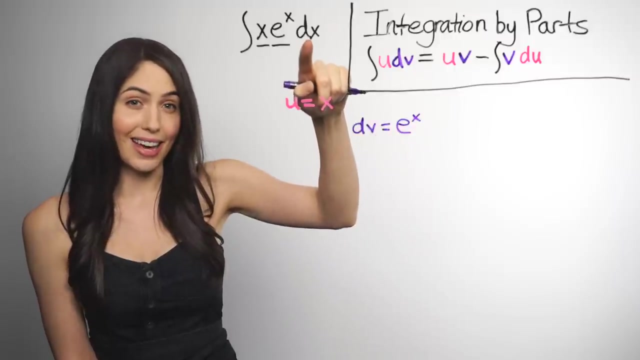 integral of that is just e to the x, which is not more complicated. So we're not in danger of that. Our dv is just the other factor, e to the x, And this is important: whichever one you pick, for dv also gets the dx, because you need that differential there. 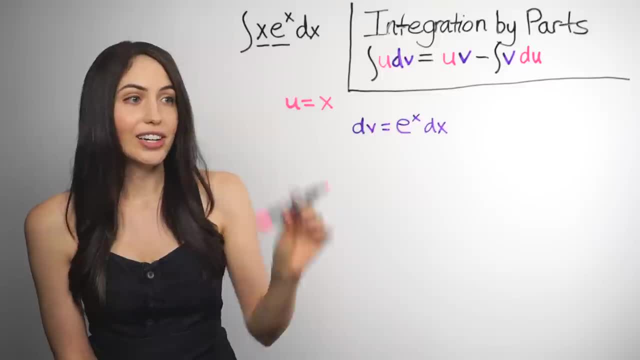 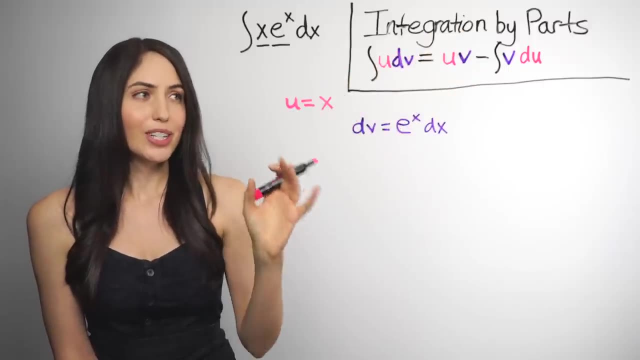 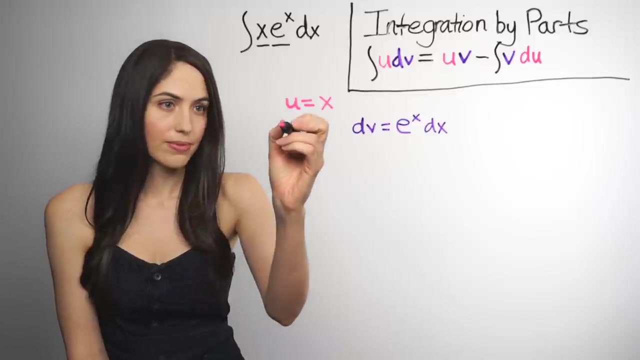 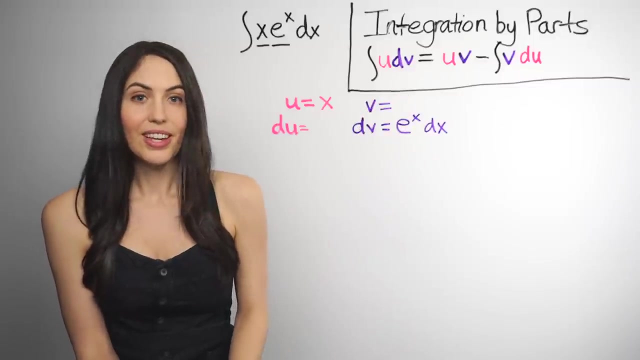 So this is great. We have our u and our dv. Now we can plug it all into the integration by parts formula. but first we do need to find two more things quickly. We have to find du and we have to know v. Okay, so we're going to differentiate u and we're going 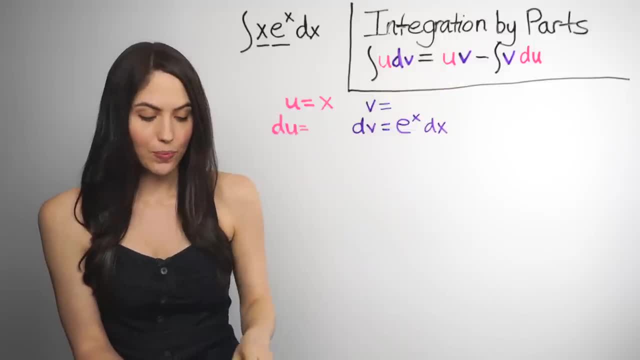 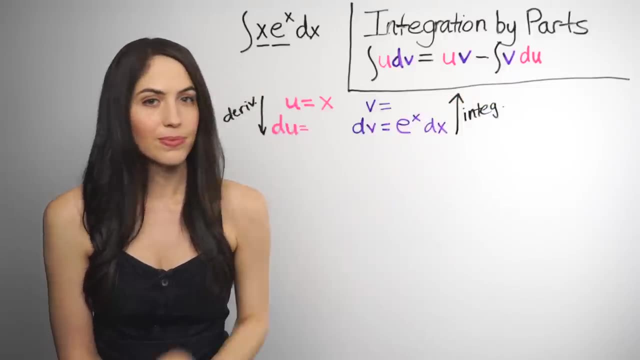 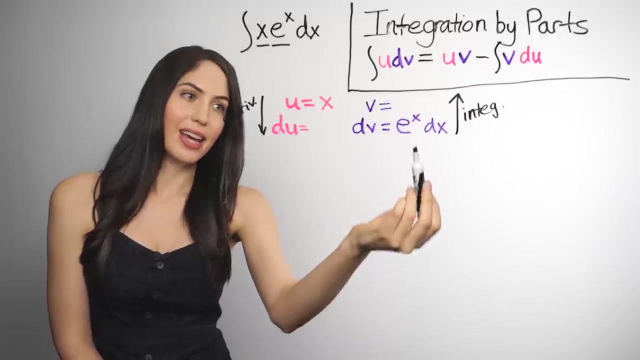 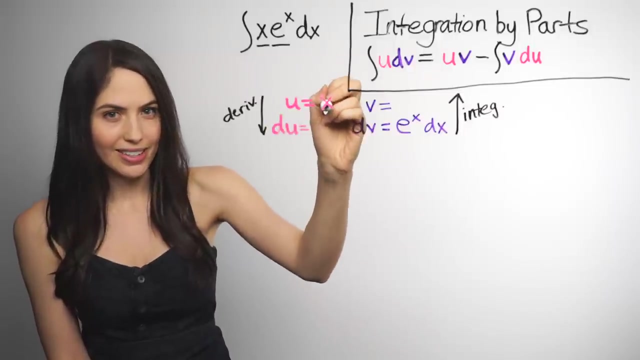 to integrate dv. So we're going to get du by taking the derivative of u and we're going to get v by integrating dv. So if you take the derivative here, we get du by taking the derivative of x. Derivative of x is just 1.. 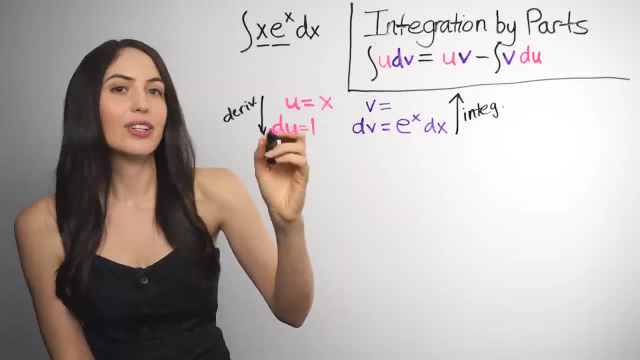 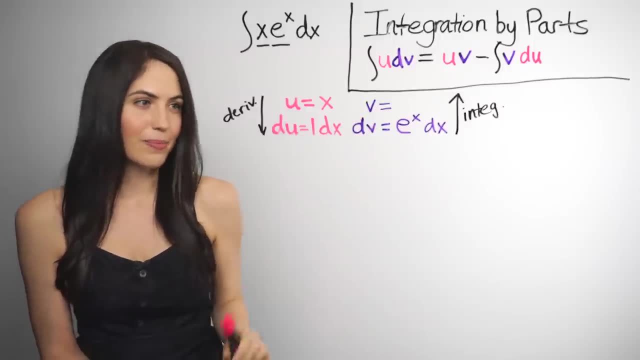 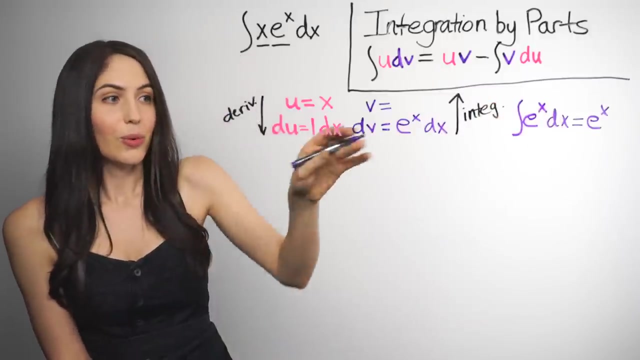 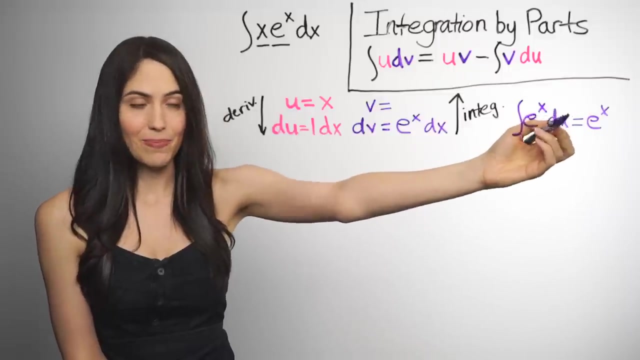 And anytime you're getting a du or a dv, don't forget the differential at the end, the dx. You need that, so don't forget that. And then if we integrate to get v, integrating e to the x is just e to the x again, So v is e to the x. And just in case you're wondering, 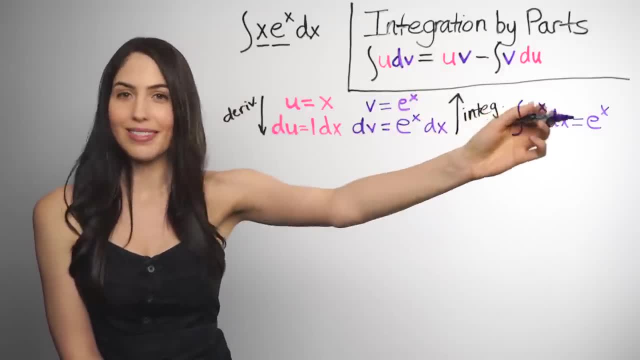 in case you're wondering, just in case you're wondering, just in case you're wondering, just in case you're a clever one. you don't need a plus c in this case. It won't matter in the end result. so you don't need to worry about writing a plus c at this point. So now, 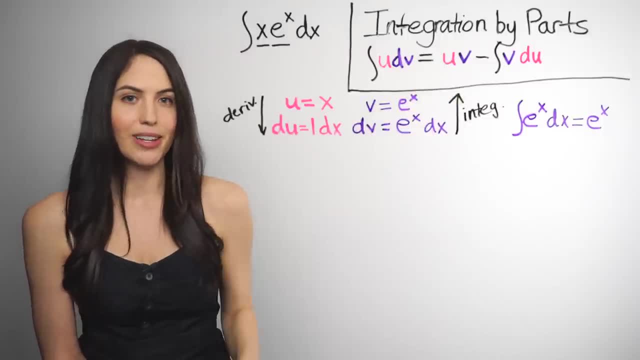 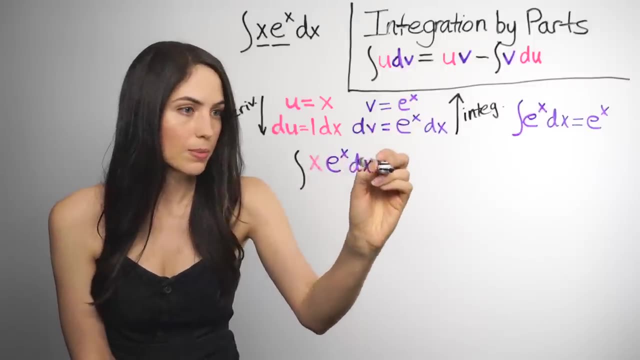 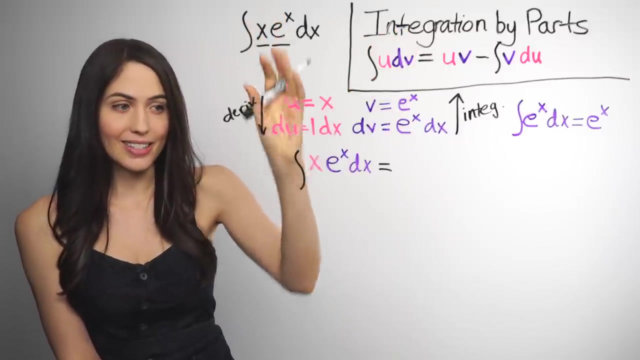 we have everything we need for the integration by parts formula so we can plug in to the formula. Okay, so now we're going to use this formula on our integral x: e to the x, dx. x is u, e to the x, dx is dx. 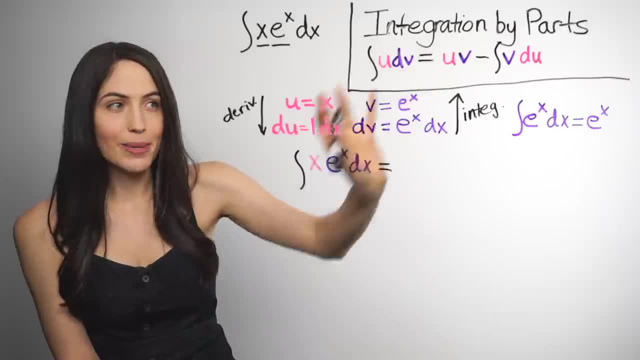 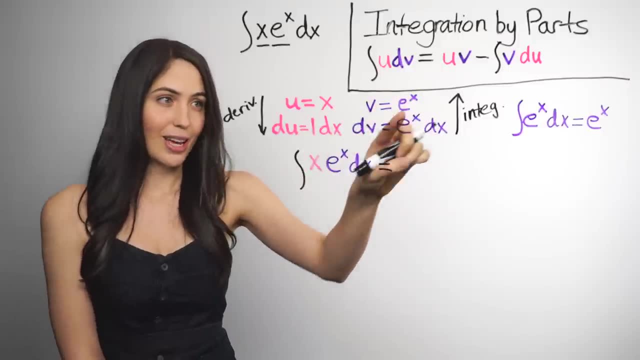 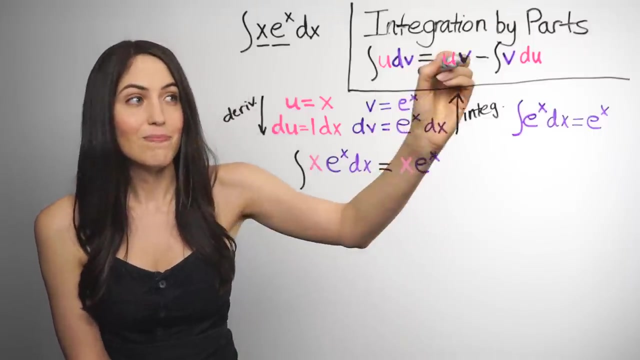 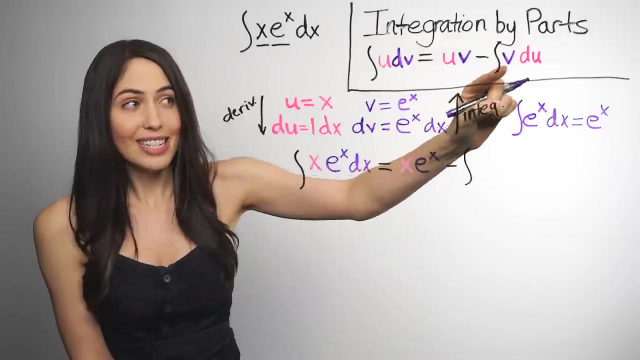 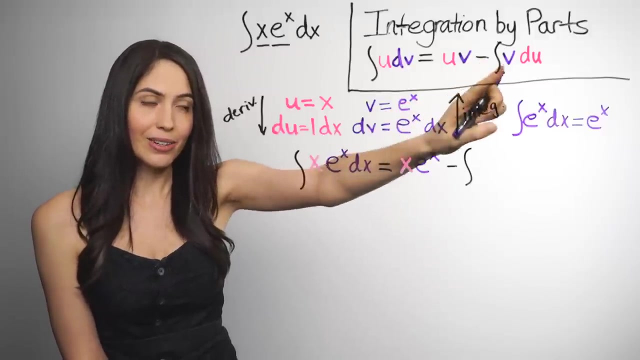 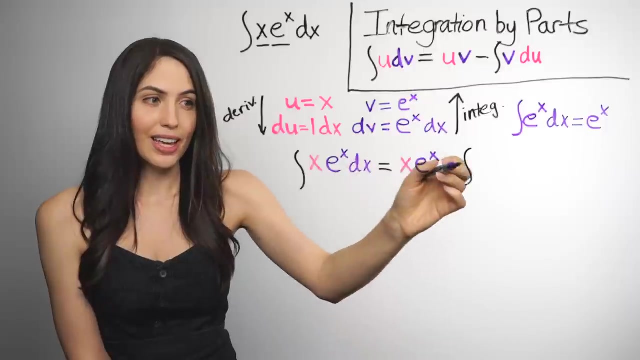 And the first part of the formula. what this becomes is first u times v, which for us is x times e to the x, minus the integral of v times du. And we have those v is e to the x 1 dx. So this is going to be minus the integral of v du, which is e to the x 1 dx, And we 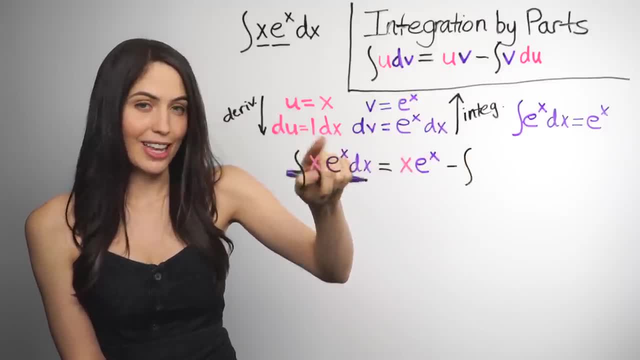 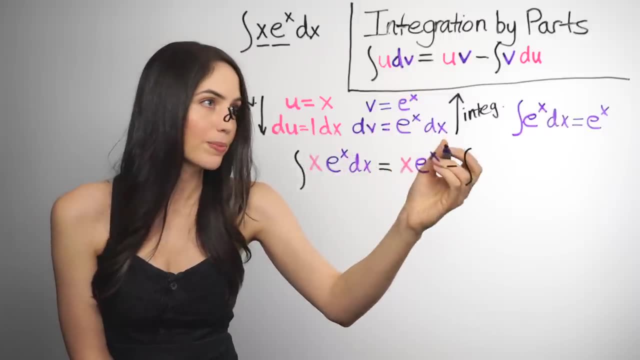 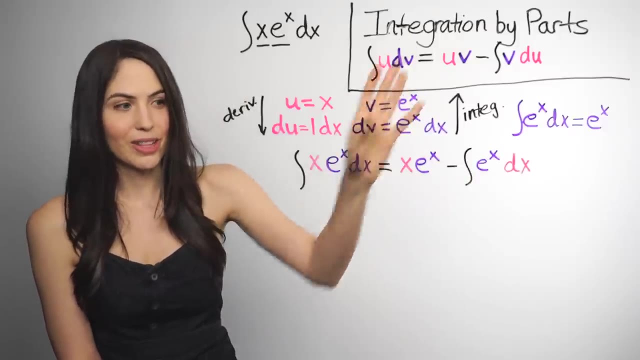 don't even need to write the 1.. This is the same as dx. The 1 is kind of implied, So it's going to be minus the integral of e to the x dx. Okay, so we've used the formula. I know this looks like it got more complicated, but it's. 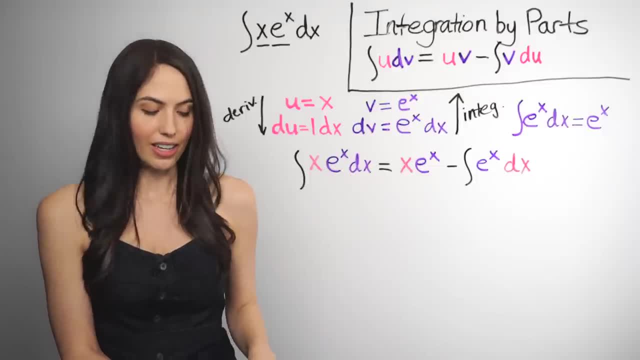 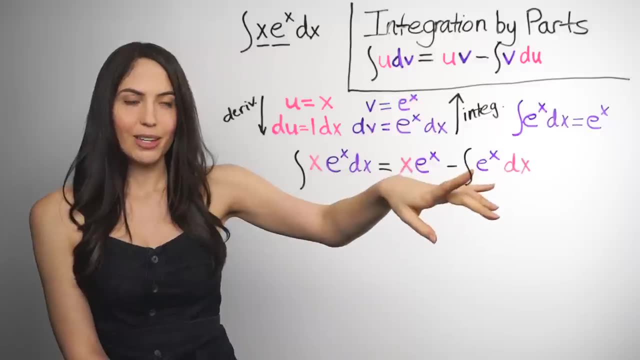 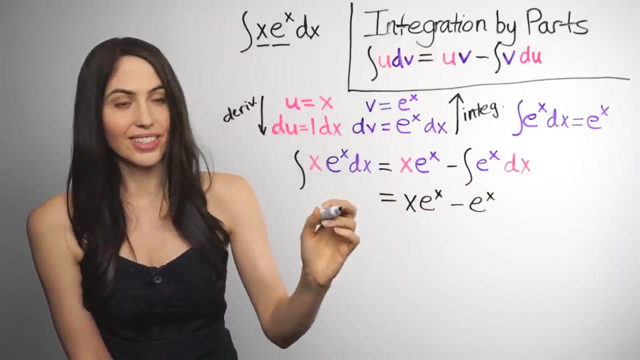 going to work out, And we're almost done, because this integral is something that we know how to do. This is an integration rule. The integral of e to the x is e to the x. So this is what we have when we integrate that. And, at the very end, don't forget to add a. 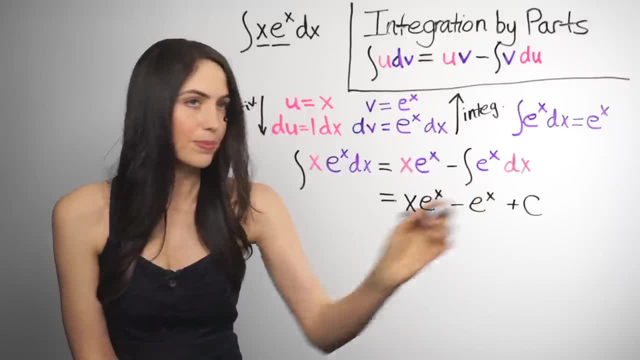 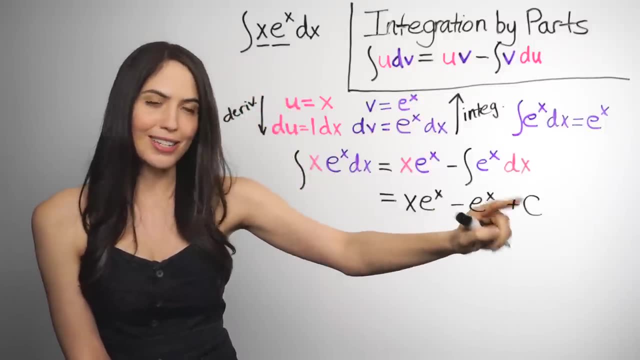 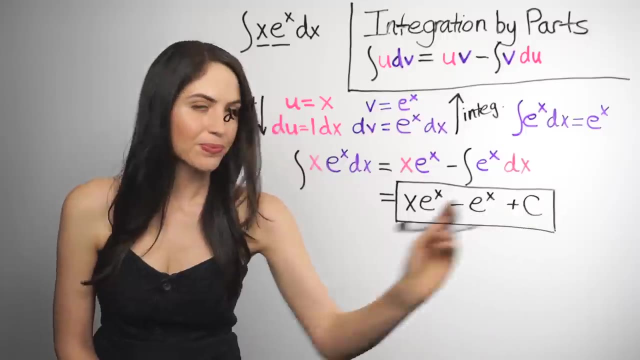 plus c. This is an indefinite integral. It has no limits here And we're going to use the definite integral. It has no limits here. So you do need to add in the constant of integration at the end. Don't forget the plus c. So this is our answer for this integral. 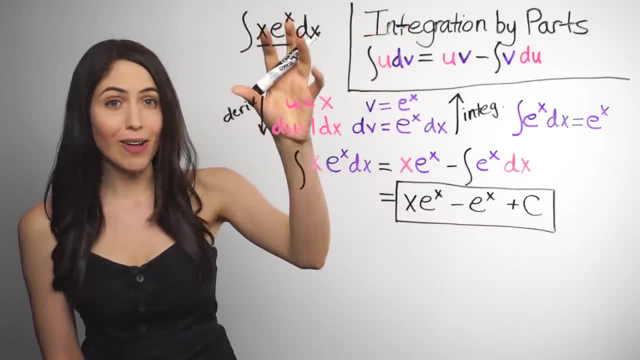 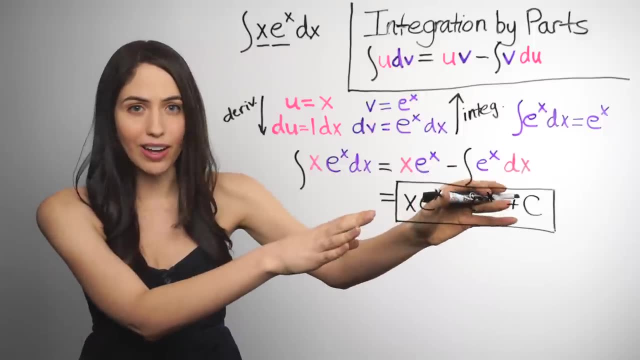 So integration by parts made this solvable, made it integrable like magic And if you want, you can check this answer. You can take what you got, differentiate it and you should get back your original integrand x. e to the x. 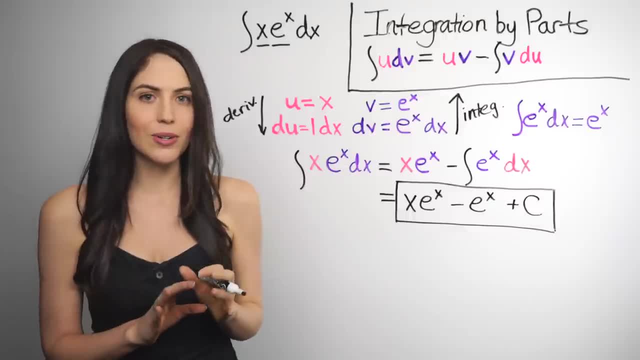 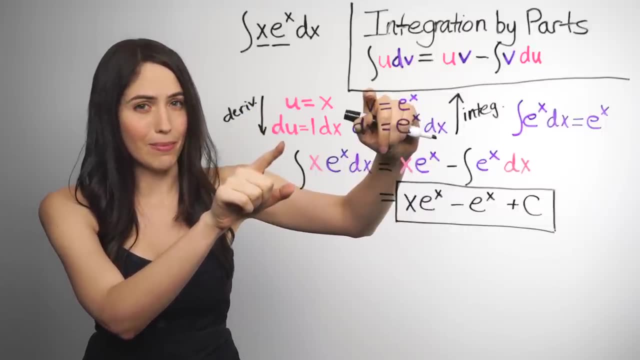 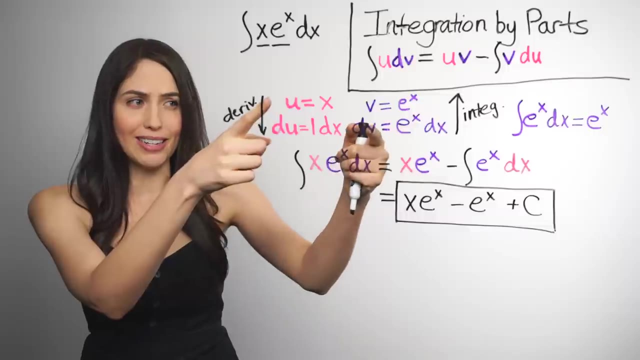 And you will. So, in summary, all you need to do is pick u and dv, find du and v from them and then use the formula. I mean, look guys, if you pick the wrong u and dv, the first. 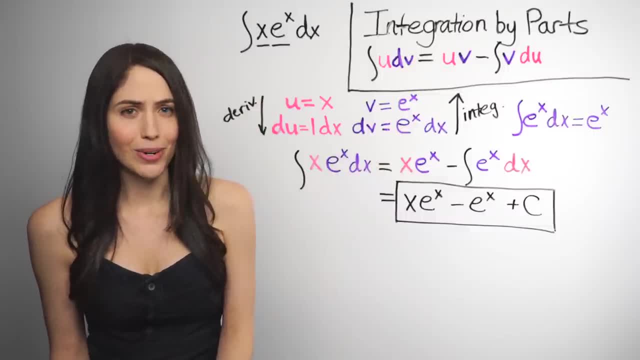 time. don't panic. It's okay if it doesn't work out the first time. If it turns out that your choice doesn't actually break it down and help you integrate, you can try something else. No harm, no foul. I have done it, and part of getting good at something is bumping up against what doesn't work. 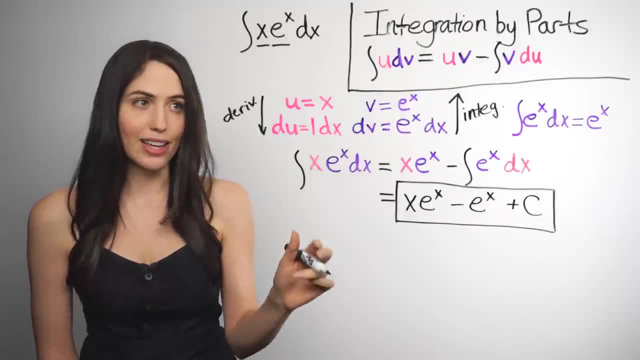 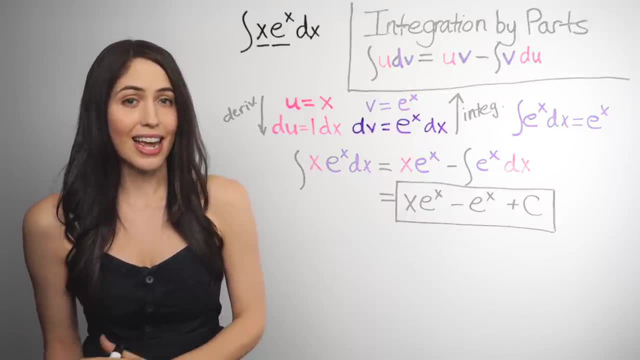 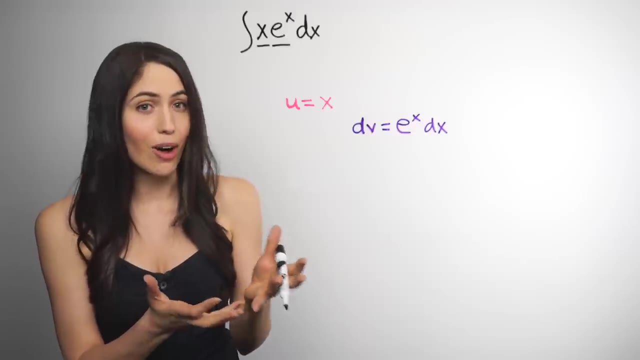 So the more practice you get with it, the more skill you'll get at picking u and dv. Ah, but you say what if you hate skills and hate developing skills and you would rather have a blind rote trick handed to you on a silver platter that always tells you what to pick for you? 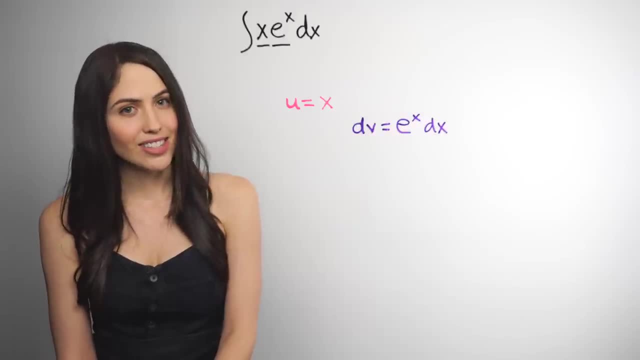 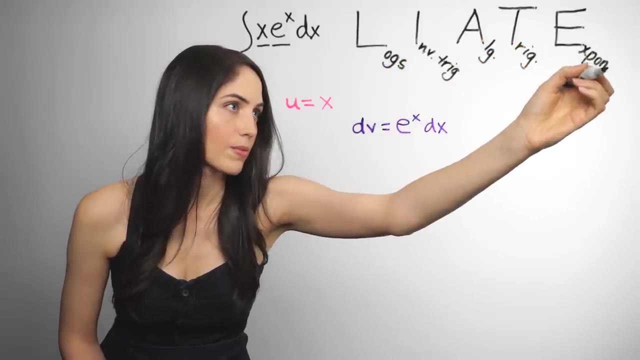 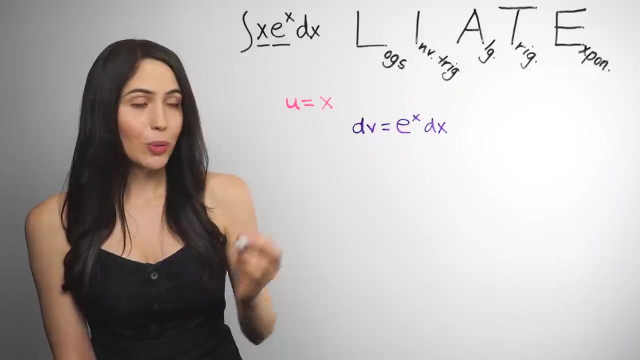 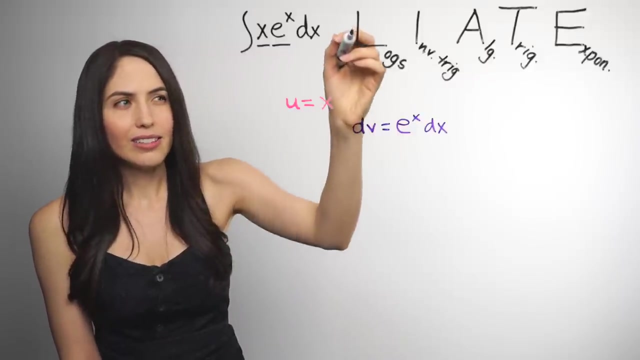 For sure. Well then, I have just the thing for you. So here's our trick. It's an acronym to help you pick u. So u will be the first thing you find in this list of letters, and dv will be the next thing you find. L stands for logs. That could be. 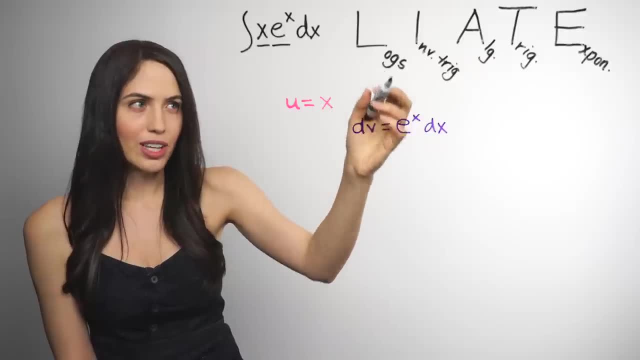 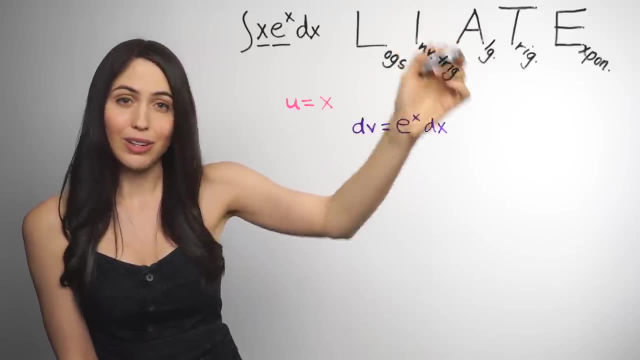 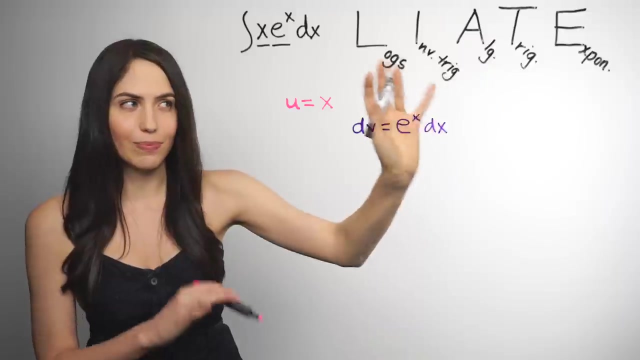 natural log ln x or normal log log I for inverse trig functions like arc sine x, cosine inverse of x. A stands for algebraic or polynomials, so powers of x, x squared, x, x cubed. T for trig functions like straight up, sine cosine. E stands for exponentials, like e to the x. 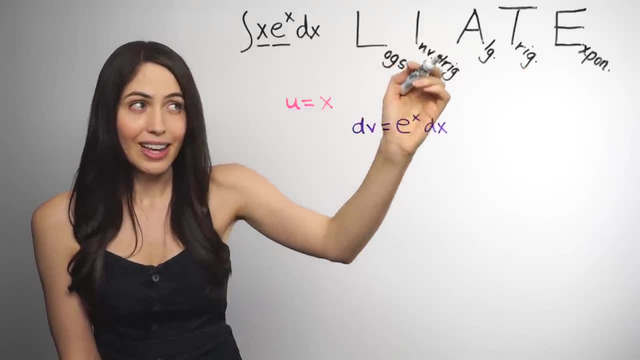 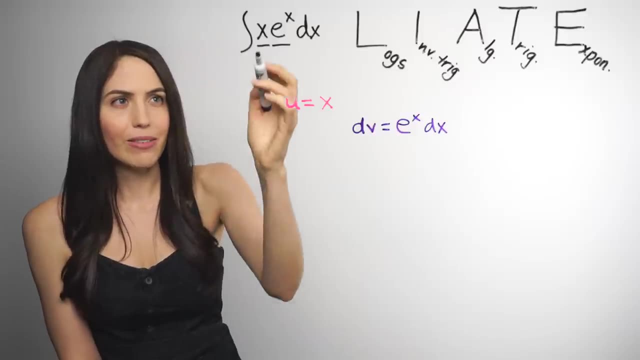 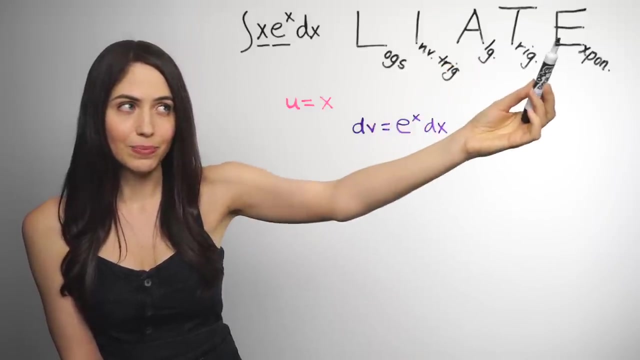 So the trick is to follow these letters in sequence, and the first one you find that you have is your u. So what do we have? We have x and e to the x. X is algebraic, e to the x is exponential. So we have a and e. 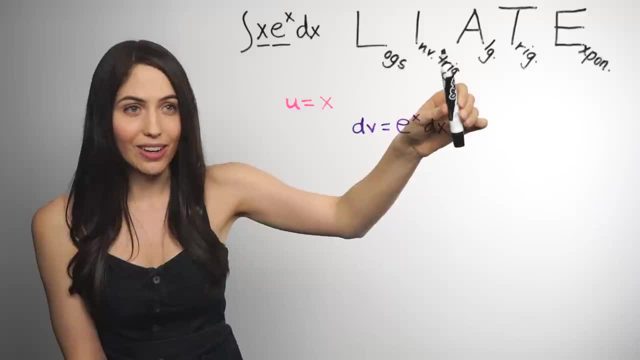 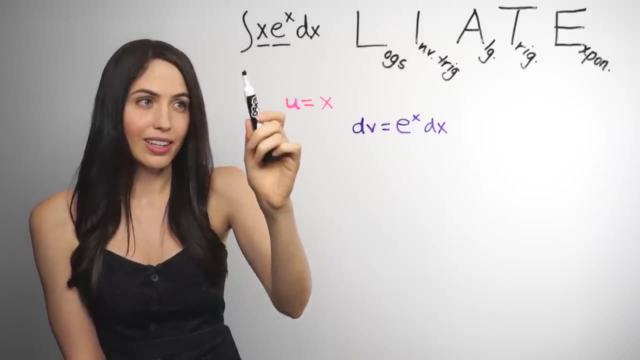 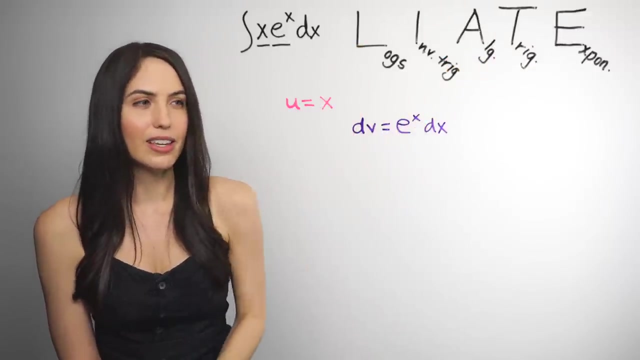 If you follow those letters in sequence, the first one you encounter that we have is a algebraic, So that x has to be our u, u is x, and the next thing we find that we have is e exponentials. So that's our dv. dv is e to the x, dx. 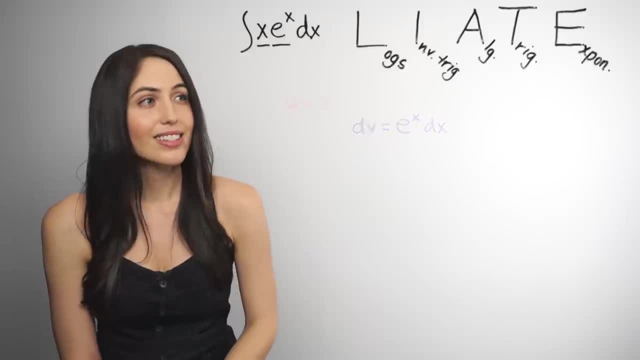 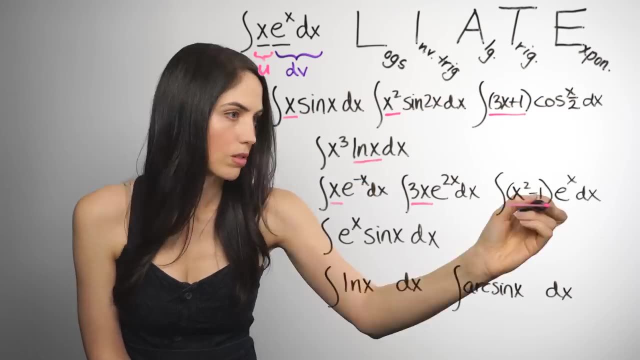 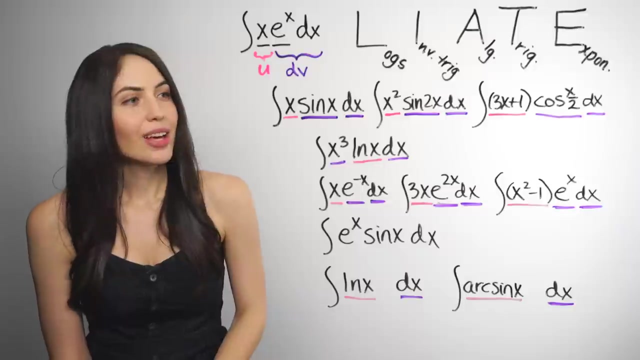 So that's the trick. It's a fun party trick. Now let's really put it to the test. Alright, look at this integral situation, Because I think the hardest part is picking u and dv. here are just a bunch of different types. 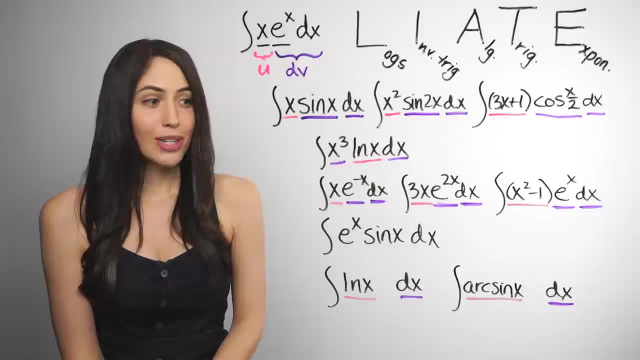 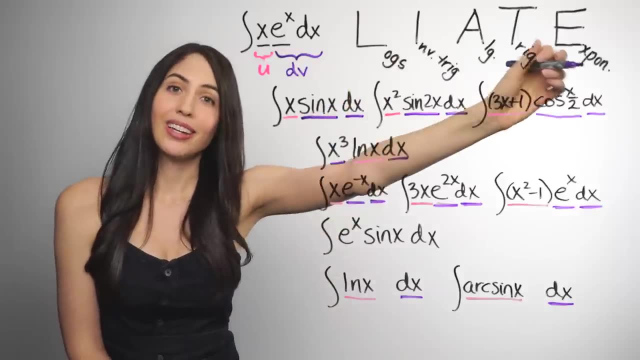 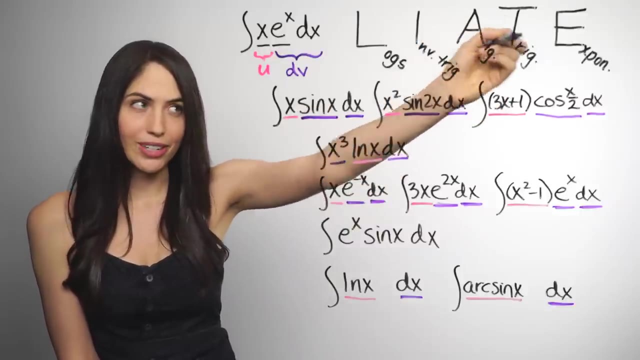 A mixed bag of types. you might see It's a real mess, so let's talk about it. Look at this one: Integral of x, sin x, dx. We can use our trick. We have x which is algebraic, sin x which is trig, since a comes before t. 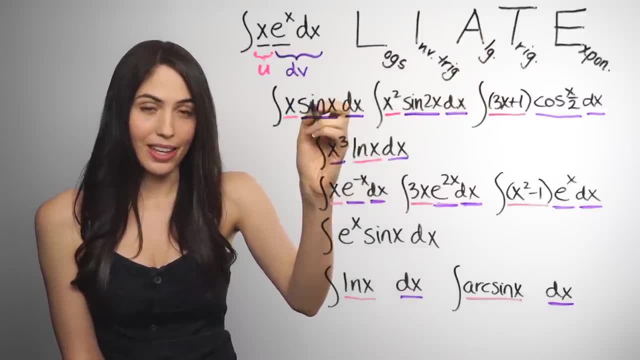 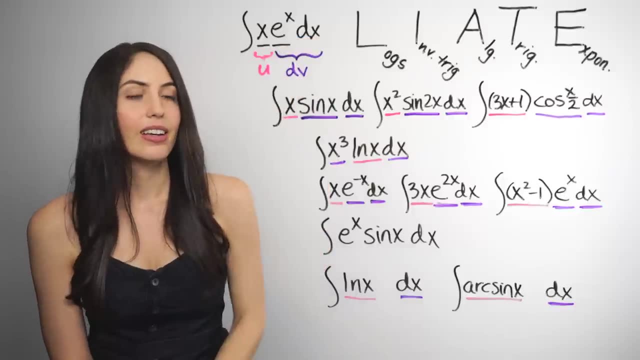 This one is our u and this is our dv. dv also includes dx, remember. So whatever you pick for dv also gets the dx, just like up here. By the way, if you didn't use the trick, it still works to think about it. 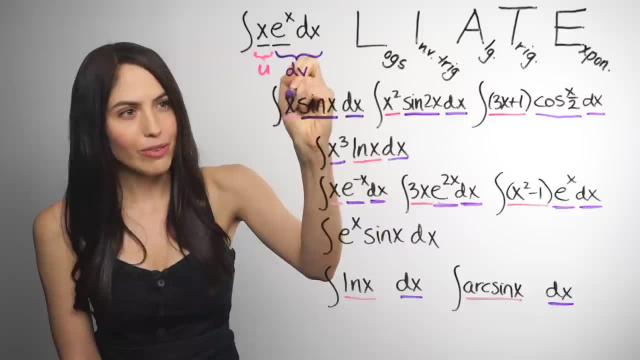 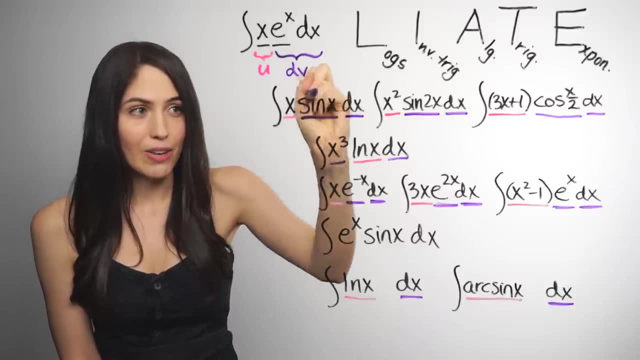 like how we were saying before: Whatever you pick for u, you want to get simpler when you take the derivative, which it does, And whatever you pick for dv, you don't want to get any more complicated when you integrate it, and this doesn't really. 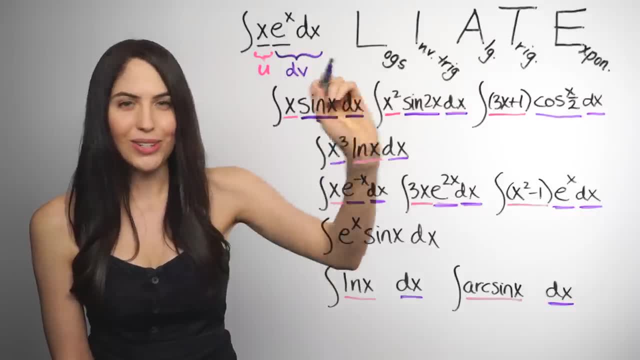 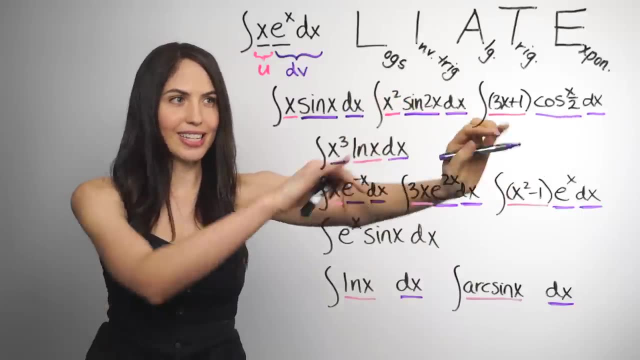 So that's why. But you can stick to the trick. These other two are kind of the same form: Algebraic and trig. Algebraic and trig. And you can see that the algebraics won out. They got placed as u because they appear first in our trick. 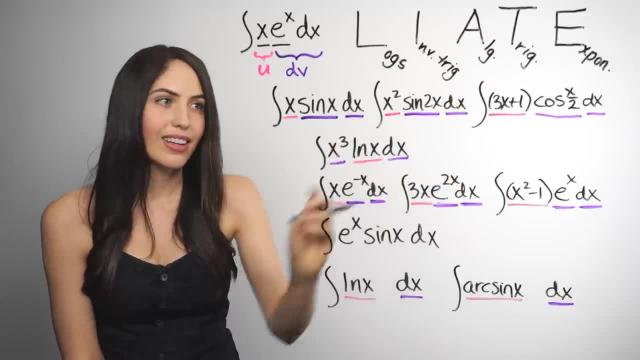 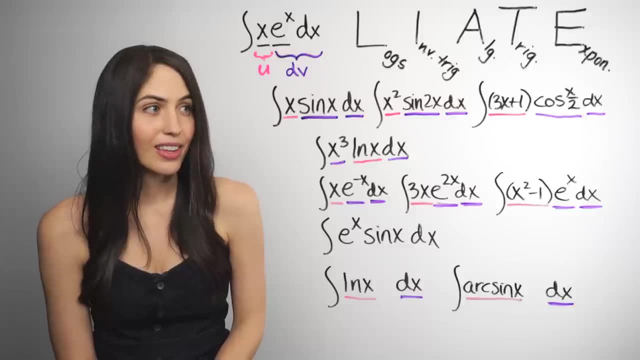 And then these are dv. The only thing I will say is that in this one you'll need to do integration by parts twice. Yeah, I know That's a whole other video, But it's exactly what it sounds like when you do integration by parts. 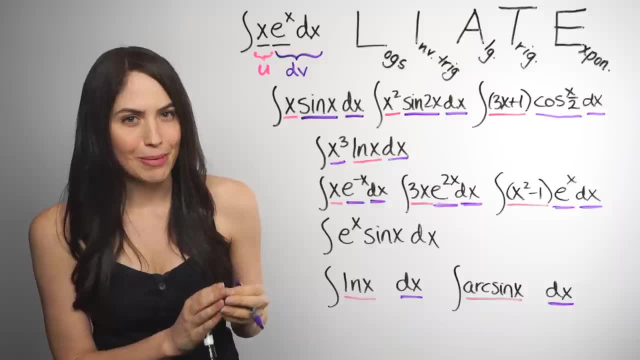 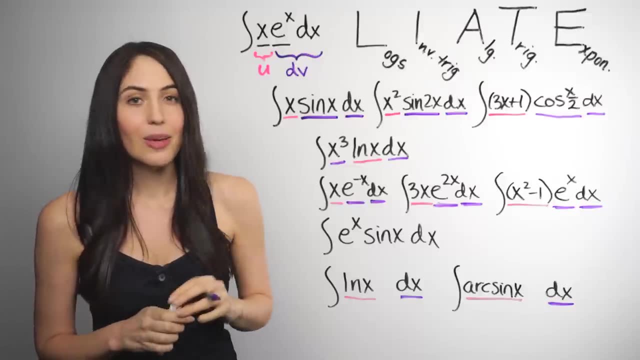 and you get a new integral. You do integration by parts on that integral in its place, And if you do that you will get the answer. But anyway, let's look at this kind, This one's here, because I don't want you to think that. 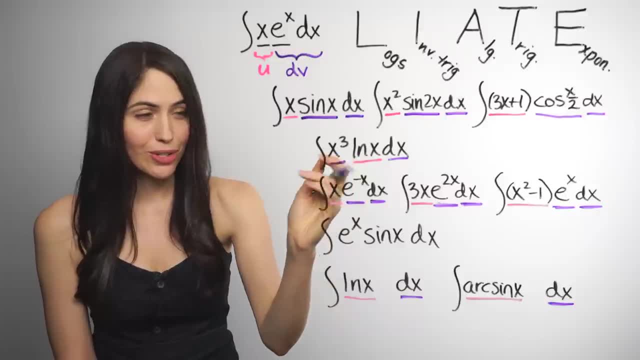 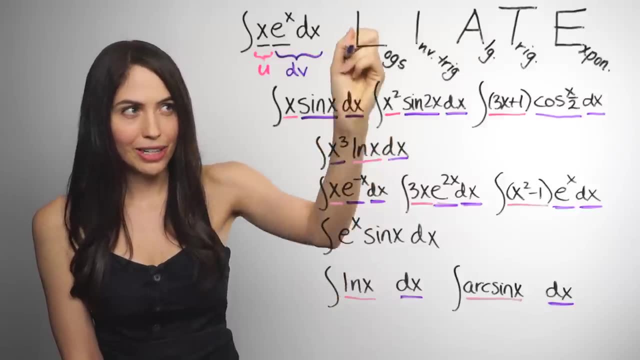 any time you see an x term, that that's going to be u for sure, because sometimes it's not Like here. Here we have algebraic and a log And, following our trick, since l comes first, our log will be our u. 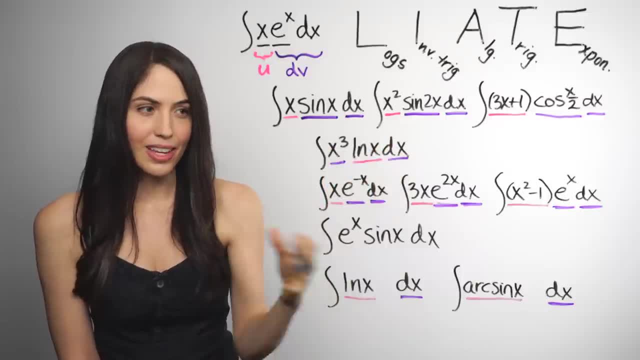 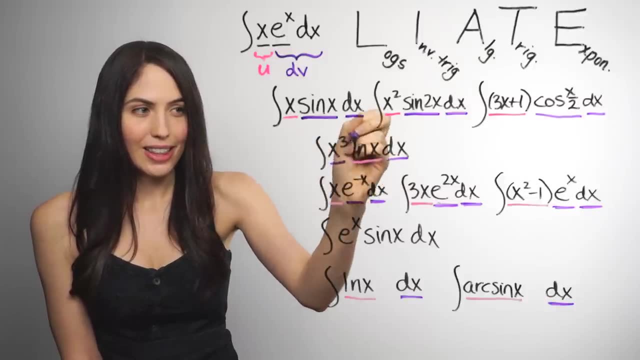 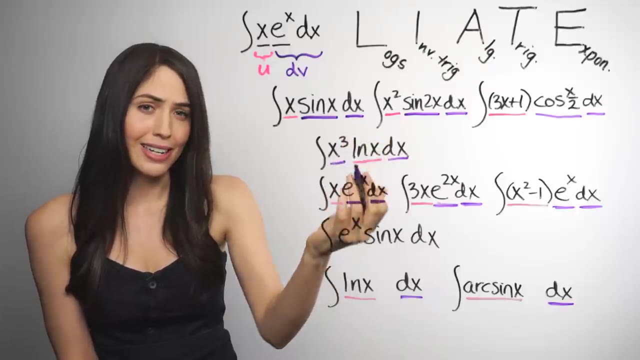 And the other part, x cubed dx, will be the dv. Okay, This also goes back to what I was saying. You don't want something to be dv if it's going to get more complicated when you integrate it- And ln definitely does get more complicated. 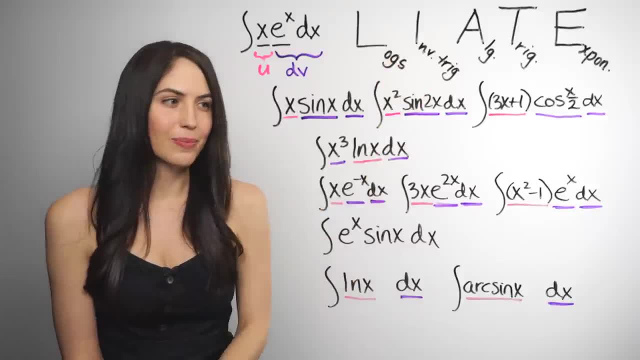 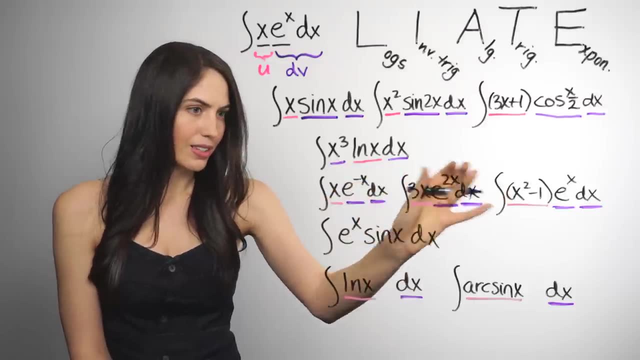 more terms when you integrate it. But you can stick to the trick as well. What about this form? We have algebraic and exponential. in all of these Algebraic exponential, Well, since we have a and e, a wins out. 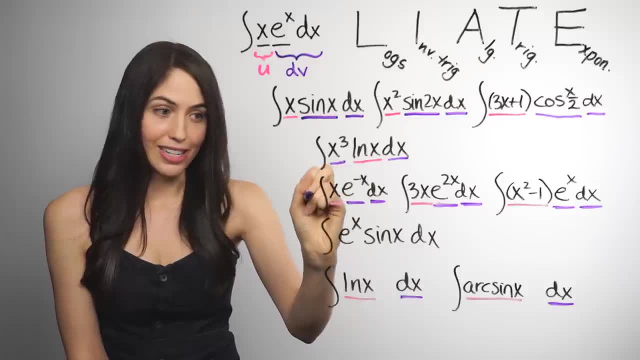 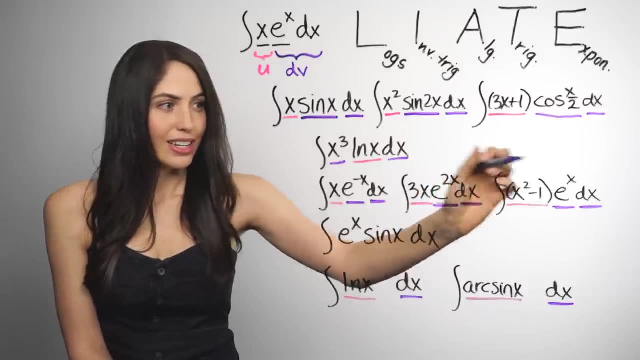 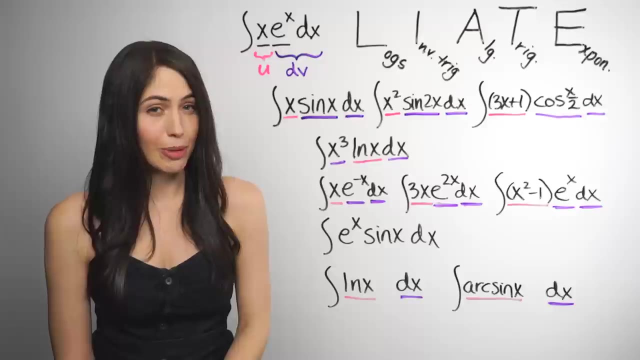 and all of those algebraics are the u's And the rest is the dv's- This one- you will need to do integration by parts twice. I can see the future. It's a very bright future- in which you need to do integration by parts twice. 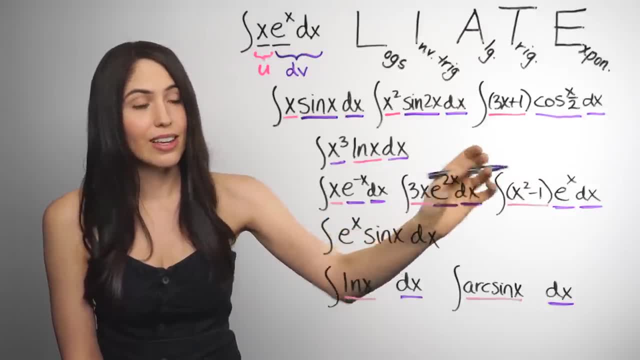 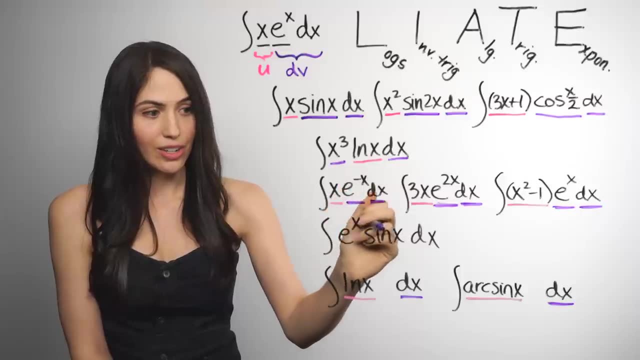 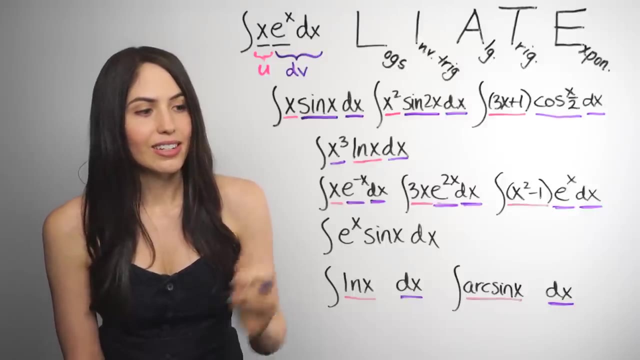 for x squared minus 1 times e to the x dx, That integral. What about this type? Exponential and trig? I haven't marked anything for this. To be totally honest, exponential and trig: e and t, e and t. 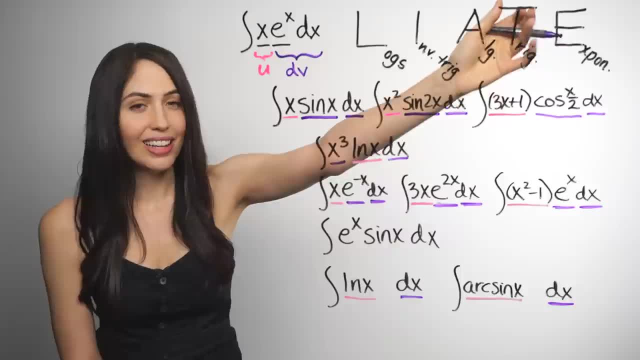 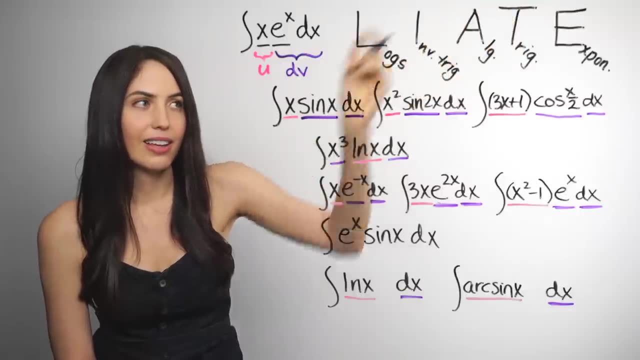 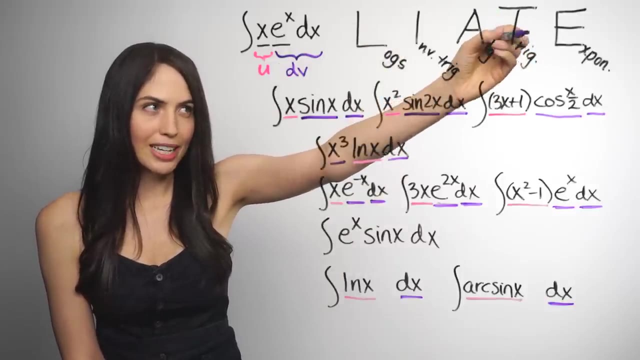 these are actually interchangeable. I lied This could be et. It's just that it would be hard to pronounce. Instead of liate it would be liate. So it's written this way so you can pronounce it, But really you can. 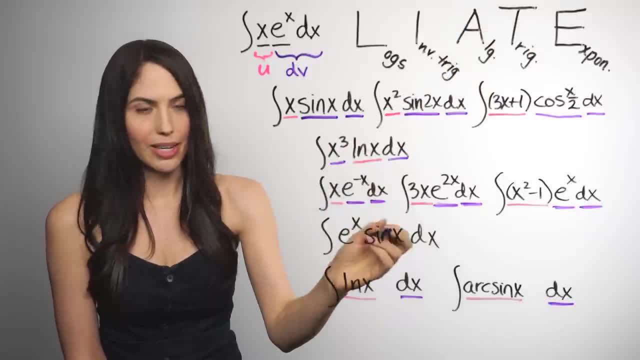 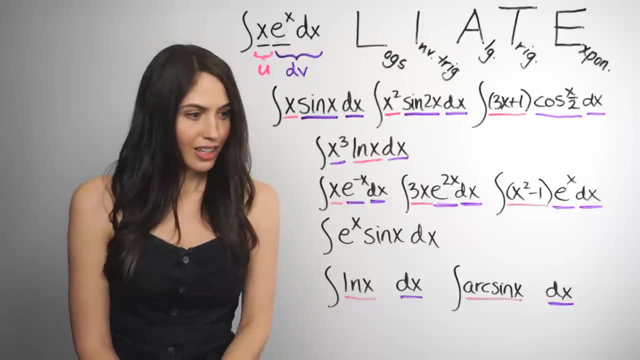 if you have only a trig and an exponential, you could pick either one to be your u and you will get the answer. It will work out. Also, you'll need to do integration by parts twice for that one. And one final kind. 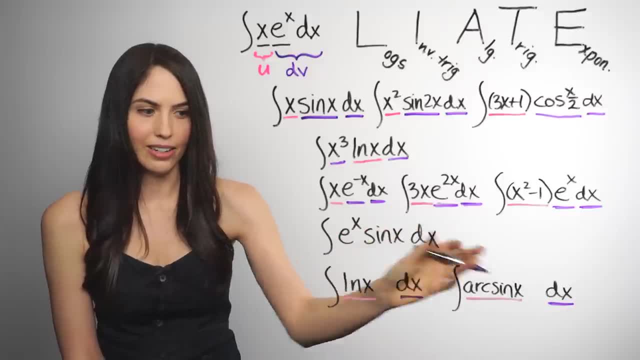 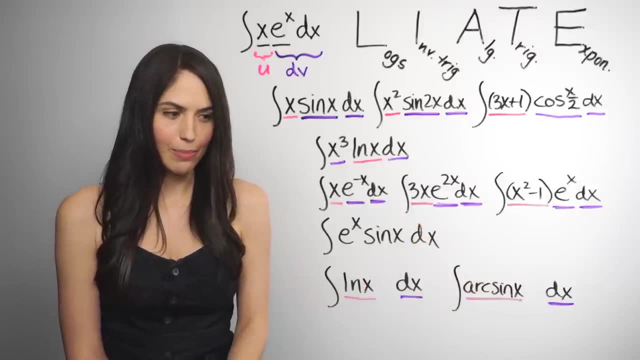 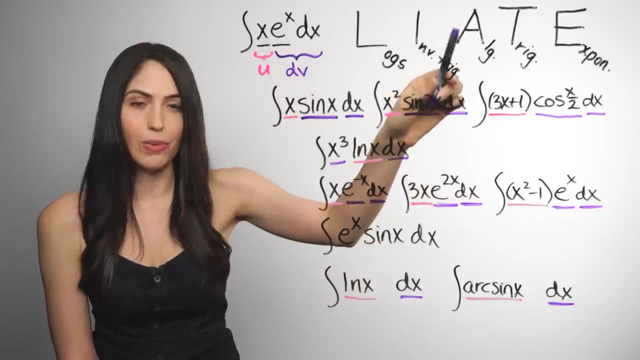 If you just have like one term in the integrand ln x, arc sine x turns out, you can use integration by parts on something like this, because the dx can be thought of as 1 dx and can be thought of as an algebraic term. 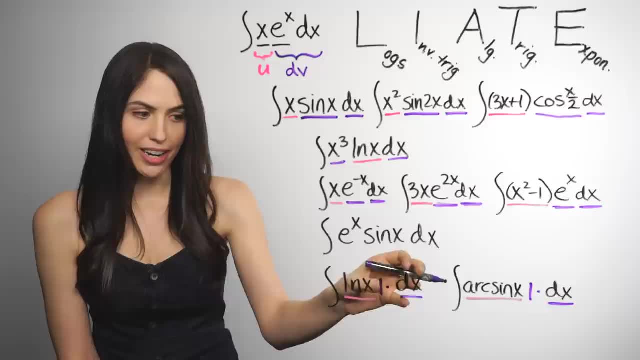 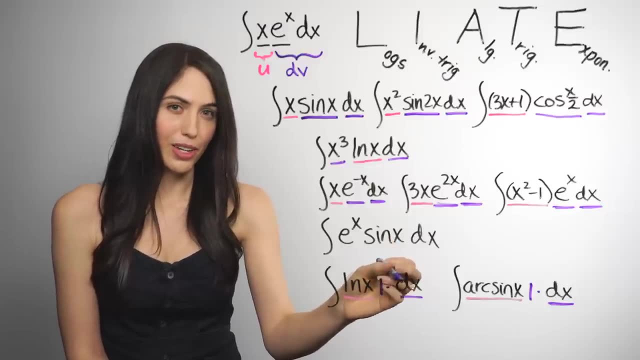 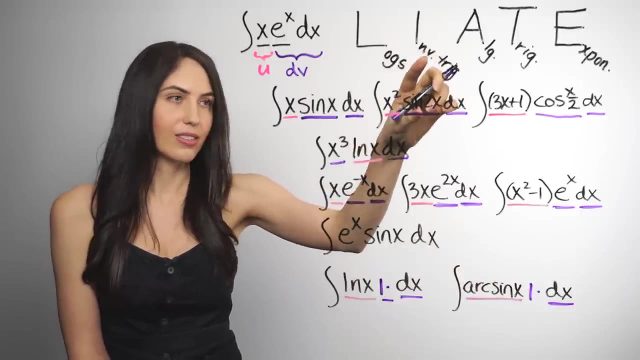 And if you do that, like here, you'll have algebraic and log. So log will be your u and the 1 dx will be your dv. Arc sine is an inverse trig, the i. in our trig It comes before algebraic, so that's the u.